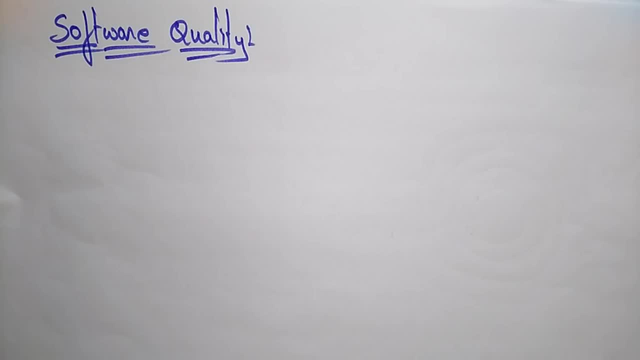 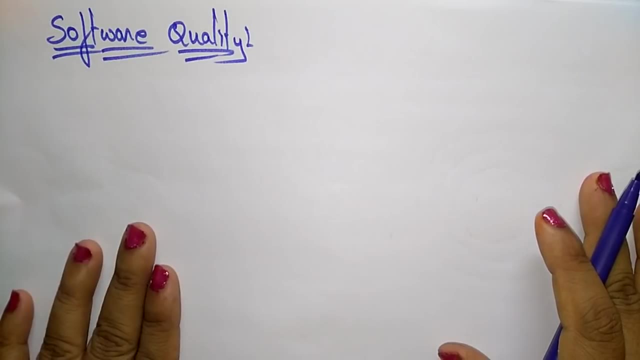 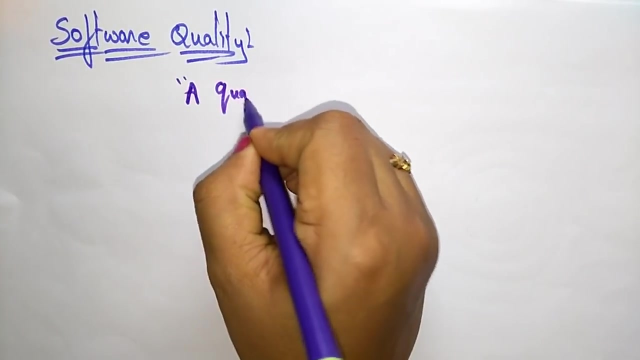 Hi students, coming to the next topic in the subject, software ensuring- was software quality. So let us see the overview of software quality. What is the software quality Actually? quality product does exact quality means, if you, the user, gets the exact output, whatever he requires, that you indicate the software quality. Let me write: a quality product does exact quality. 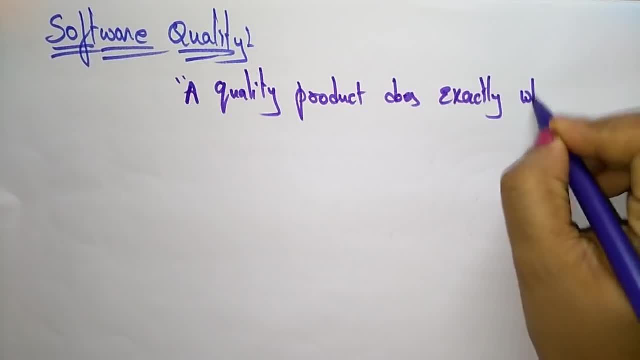 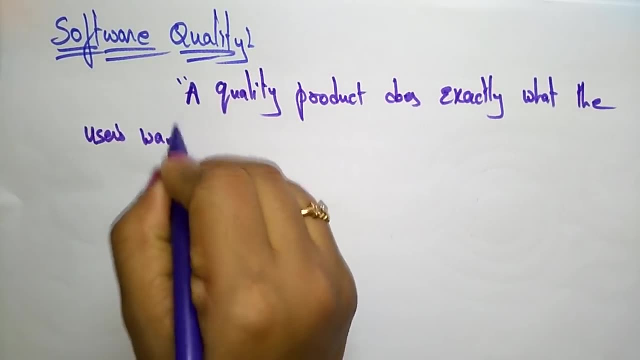 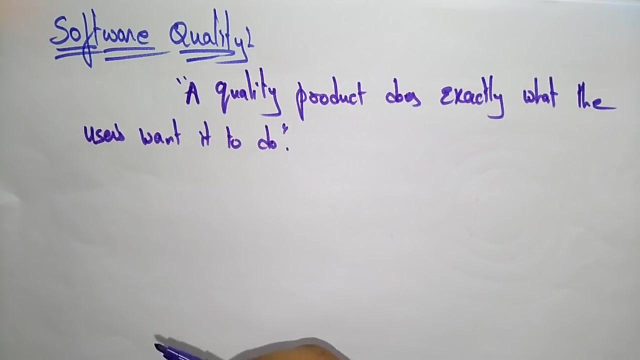 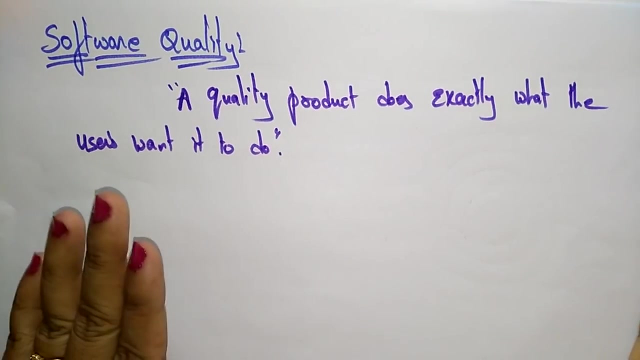 Exactly what the user wants it to be. what the users want it to do means wanted to do. Suppose if the product was that if the user want to do something, if he is satisfied with that, then you can say that the software is a quality, a quality product. a quality product does exactly what the user wanted to do. 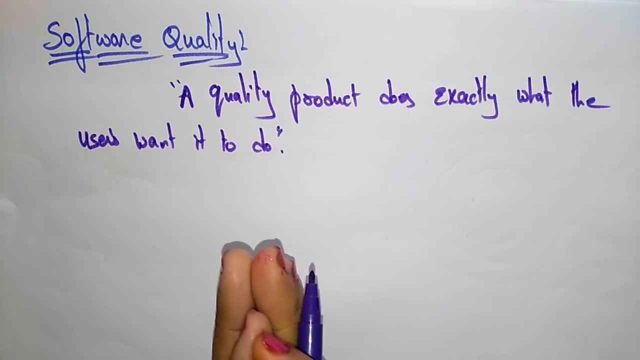 So let us see the software quality. So let us see the software quality. for software products, the fitness of purpose is usually interpreted in terms of satisfaction of requirements. so that thing, you have to be remember that. so always the software products, the fitness of purpose is usually interpreted in terms of satisfaction, the satisfaction of a requirements. 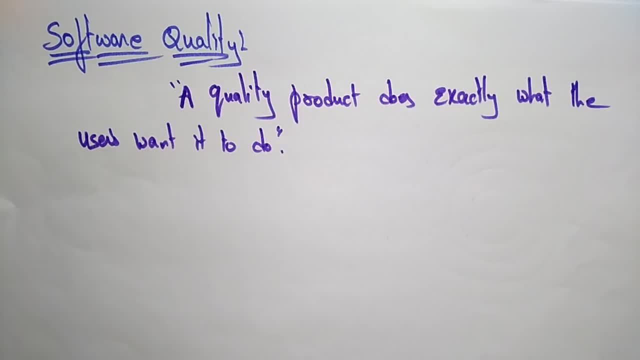 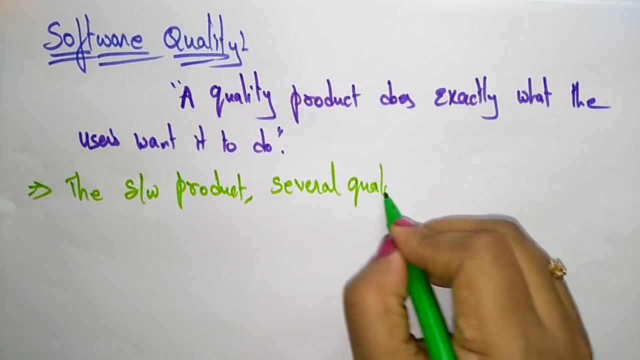 now let us see some of the software products. uh, that's several quantity factors. so, whatever the software product you have taken, software product, several quality factors. so what are the quality factors that are present in any software product, whatever the software product you have taken, and what are the quality factors that will be present? 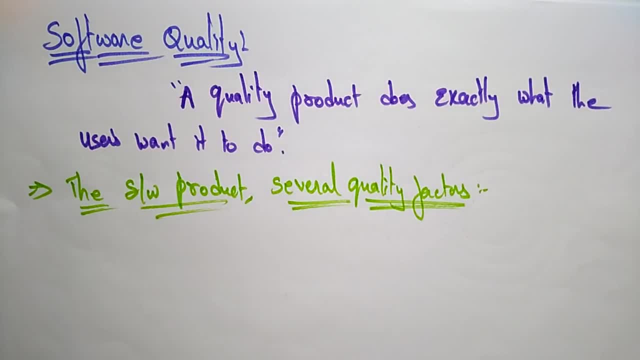 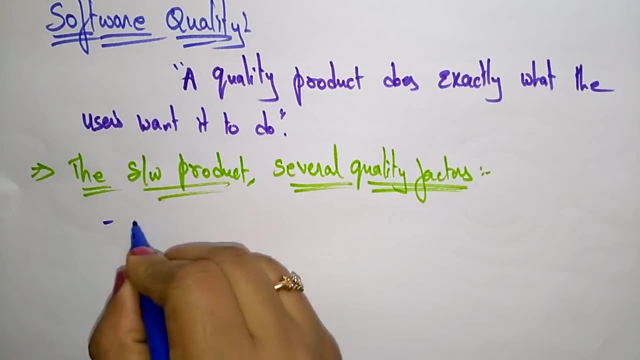 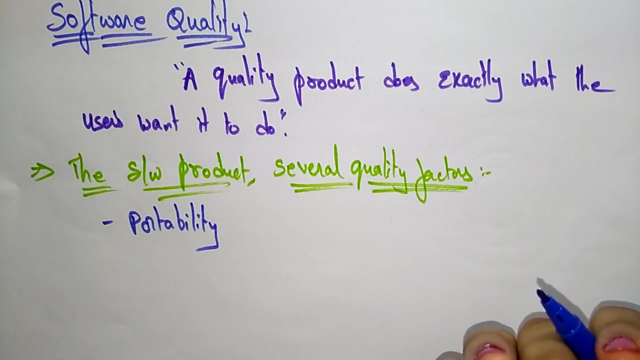 on that software product, what terms? you can say that it is a quality product. so those software qualities or portability, if your software product is portability, then you can say it is a quality product. portability means it's a platform. independent means it has to work in different operating. 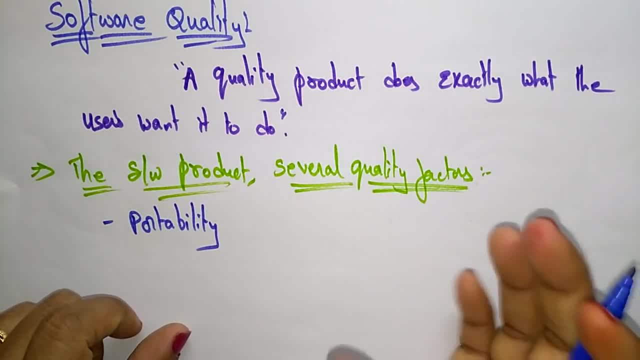 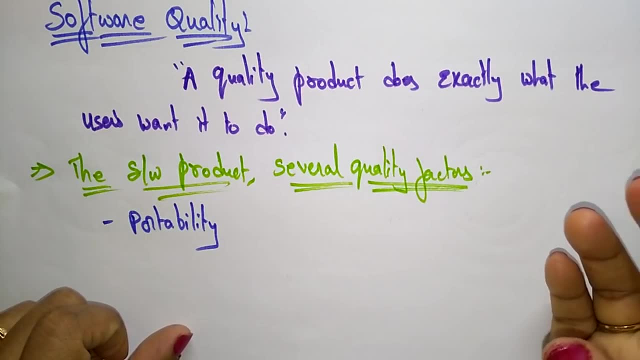 systems. so whatever the operating system is there, that in your system, your product is going to be work in that operating system and whatever the different machines, also it going to be supported. different apps are going to be supported. it means the product is used using any way. that is a portability. so the first quality factor is it should be a portability.